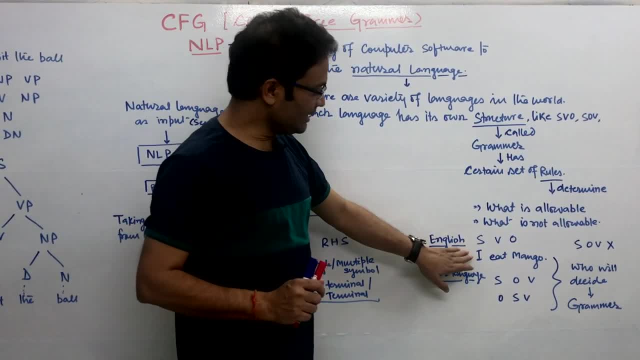 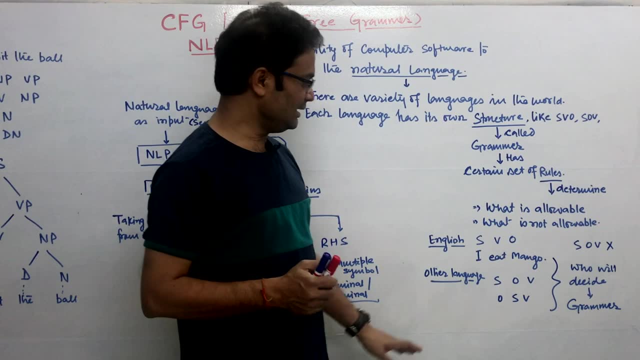 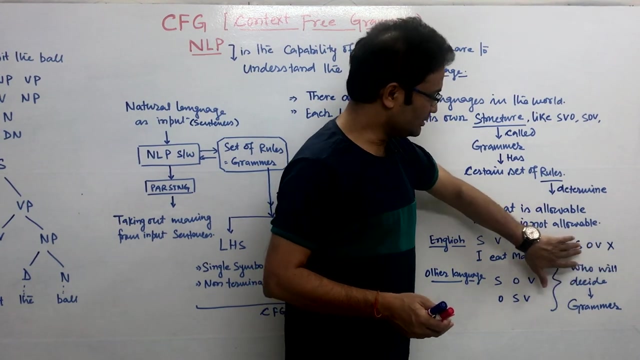 So take the example of the English English. if I say sentence I eat mango, here is the subject, verb and object. I cannot say that I mango it. we can't, we cannot go for the subject, object, subject and object and the verb. 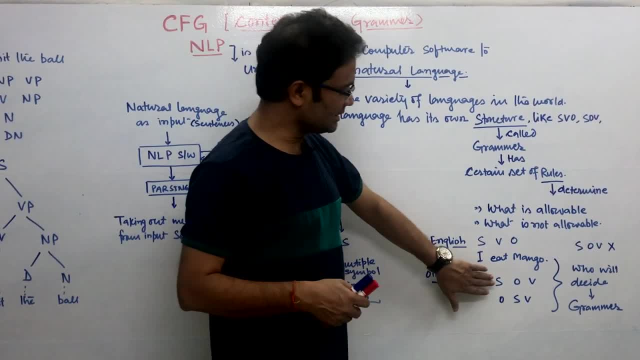 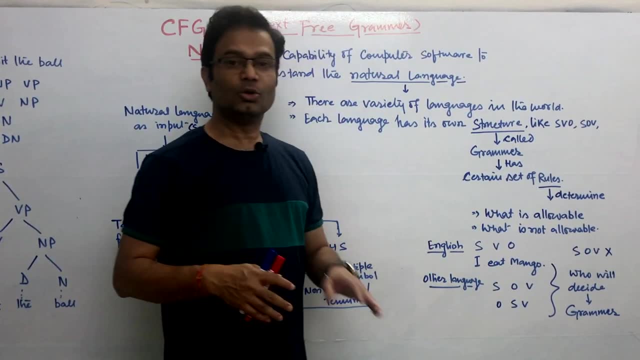 But if you take the other language, we could have the subject and object and the verb and different languages. you could have the object, subject and the verb. So who is going to decide? which is the set for the English, which is set for the different? 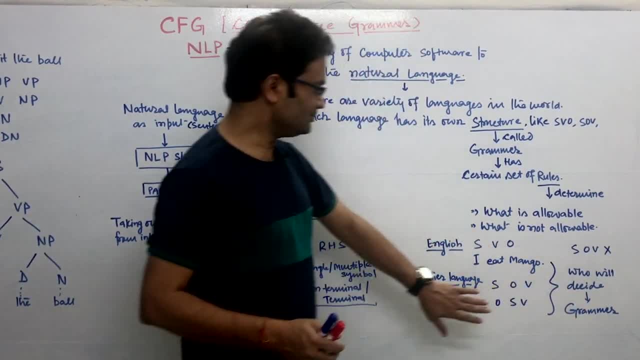 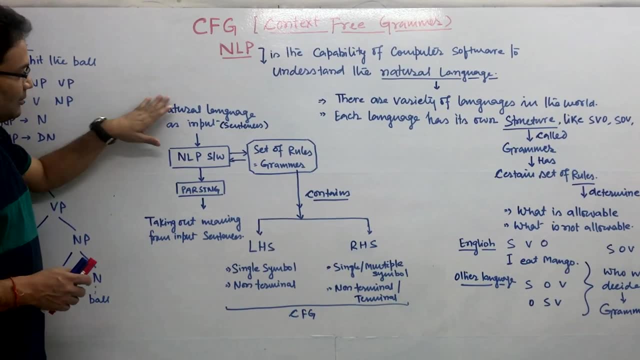 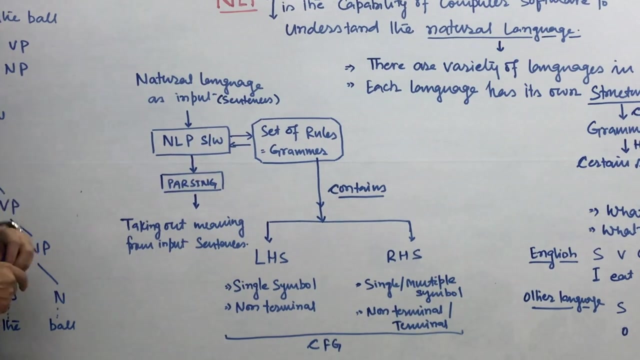 language, and that is nothing that is called the grammar. Ok, Okay, so the same thing we can understand again with the help of the pictorial diagrams. So suppose we have the one natural language that is the input for my NLP software. So what this NLP will do with the help of the grammar set, of the rules or the grammar. 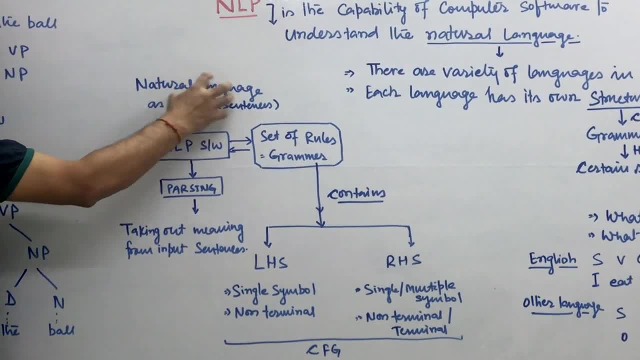 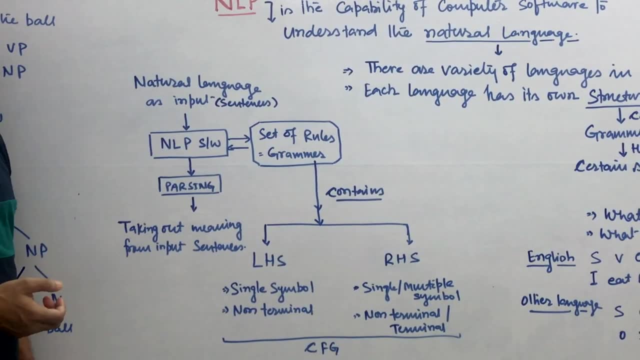 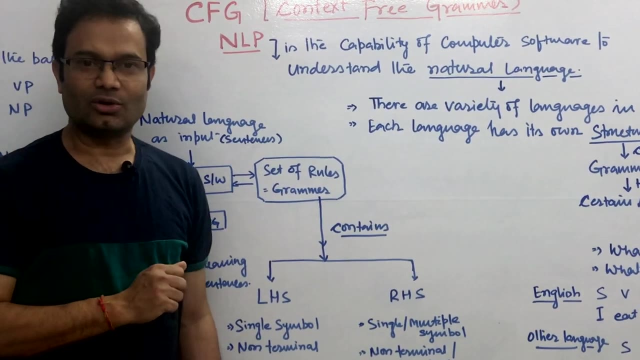 as you can call. they will take the input sentence. with the help of the grammar they will parse your sentence and that is taking out the meaning out from the sentence. So suppose if I say to my computer: hey, computer, I want to listen this song. 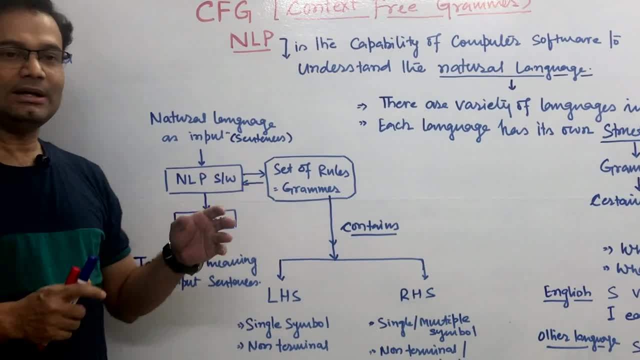 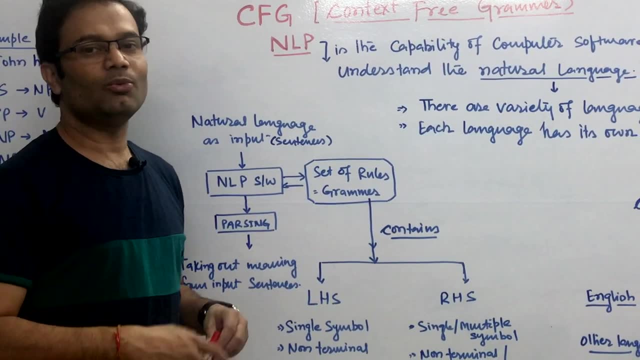 So first computer will check, with the help of the NLP, my sentence is correct or not. So they will do the parsing and after parsing they will take out the meaning what the sentence I had given. right. So now if you see what is the rules. 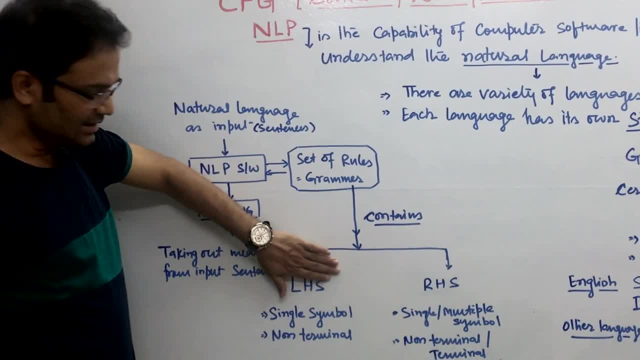 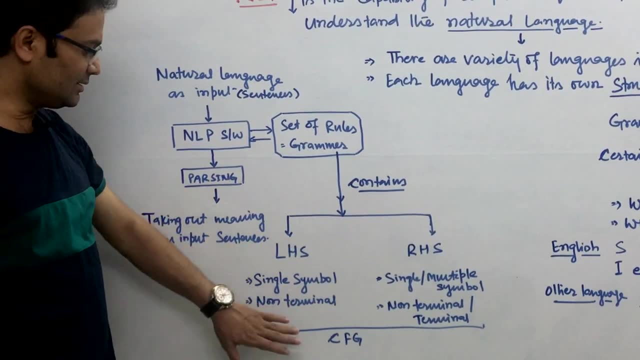 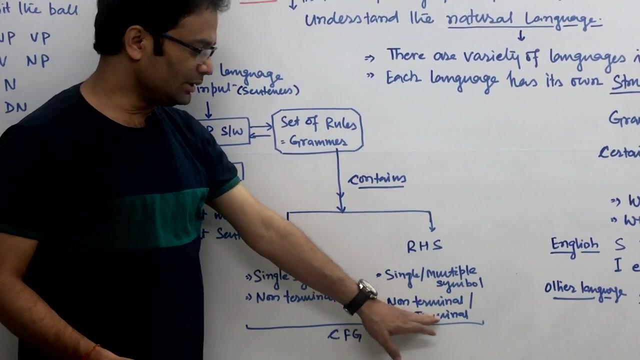 So this rules contain the two part. one is the RSH- left hand side, one is the RSH- right hand side. RSH part has always the single and that is called the non-terminal and right side. we could have the single and multiple. we could have the non-terminal and terminal. 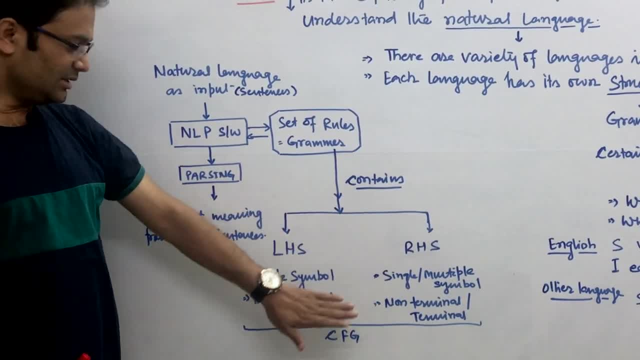 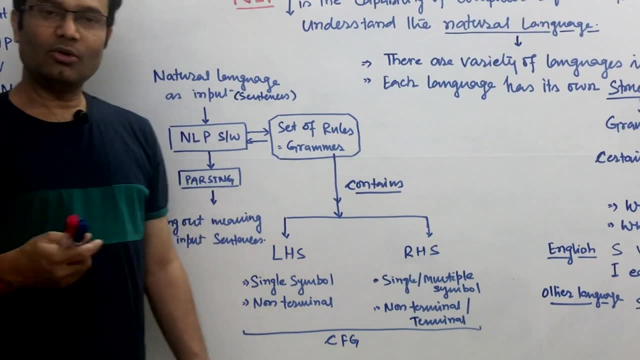 Do not worry, I will explain each and every context in detail. and this complete thing is called the CFC. it is called the context figure number. Before going to the definition- Okay, Before going to the definition of the CFG, let us have one glance how it looks like CFG. 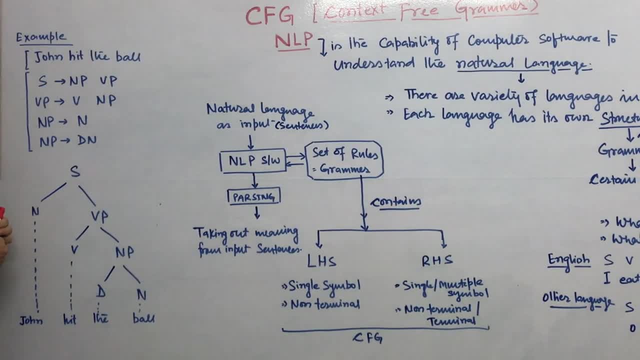 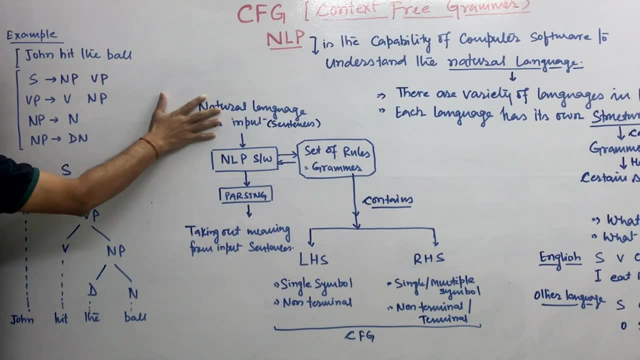 right. So I made one example here. So suppose if you have the one sentence, John hit the ball. This is the given sentence, natural sentence, right, And this is the set of rules. there is nothing. this is the set of rules. 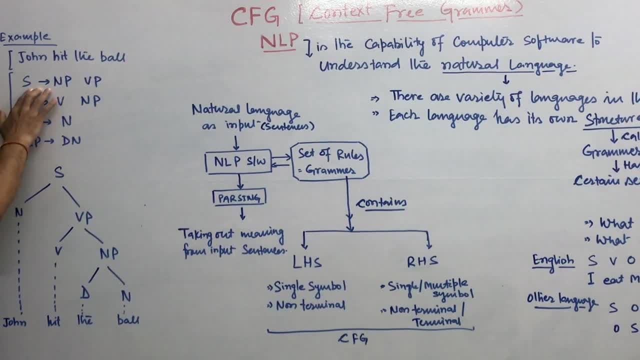 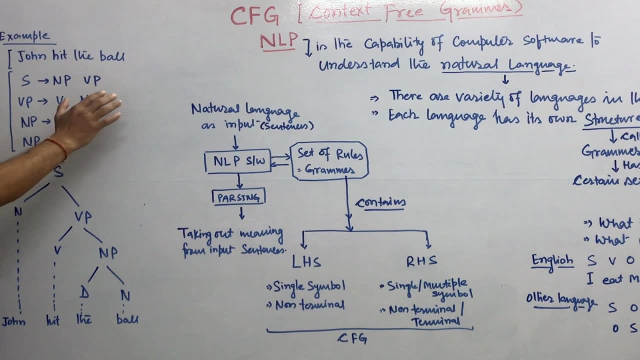 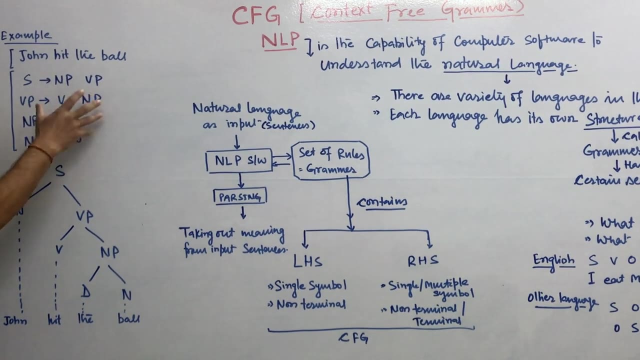 So what is the rules? Any sentence in the CFG start with the starting symbol and they could have the noun phrase and the verb phrase. Verb phrase can further divide into the verb and the noun phrase And this is the. we will discuss more about that, but just for time being this is the. 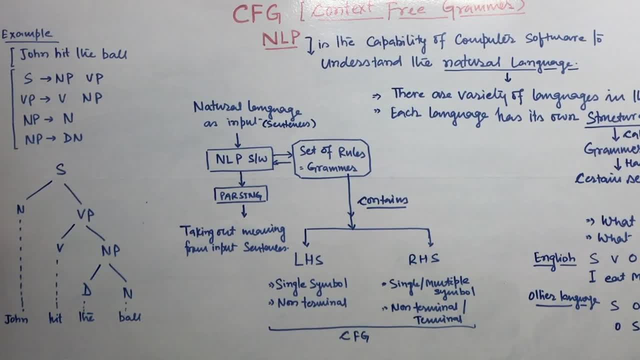 set of rules and this is called the RSH part. So, if you see, this is the complete RSH part. they have always the single, one single symbol and this is called the RSH part. they will have the one or more than one symbol would. 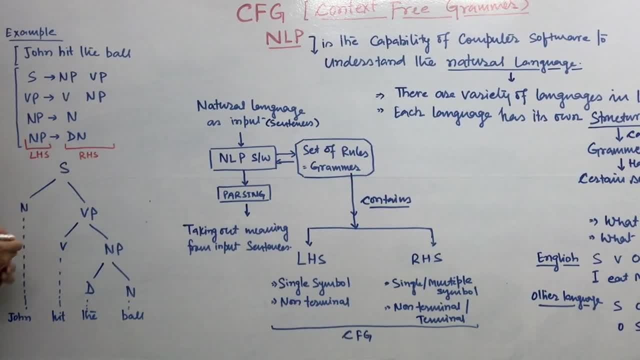 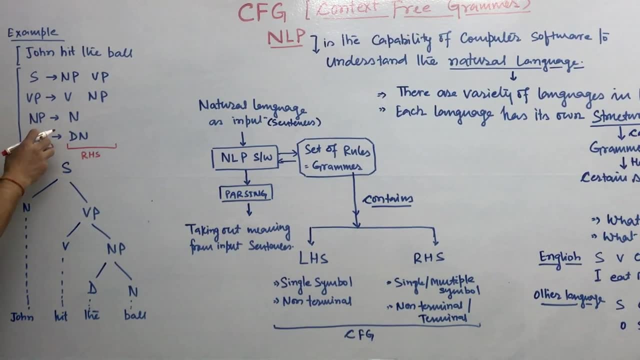 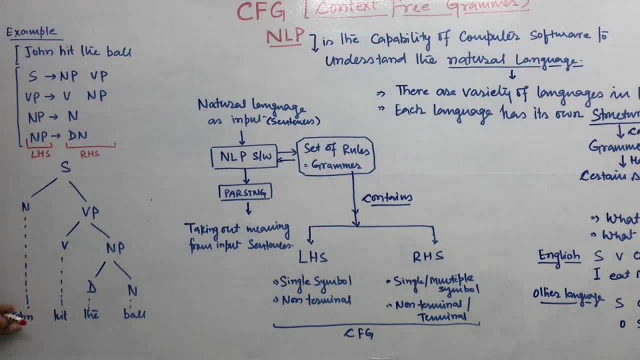 be there. And few symbols is called the terminal, few symbols is called the non-terminal. So RSH side is always the non-terminal. Non-terminal means they can further divide it into the terminal right And this is called the terminal. these words: 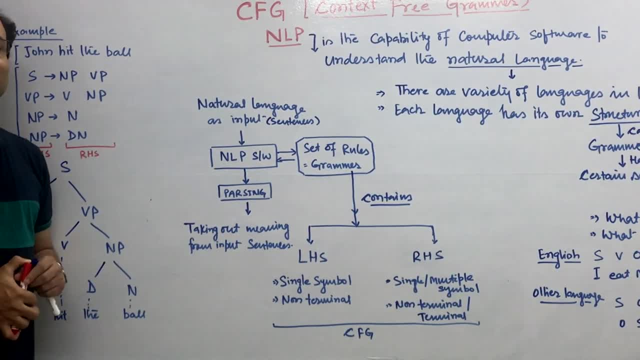 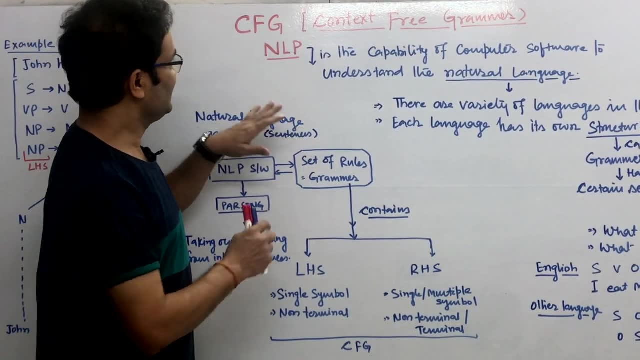 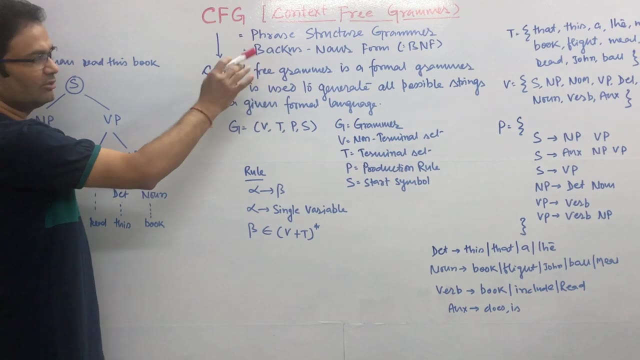 So terminal cannot further divide and terminal belongs to the word vocabulary, actual word, ok, So now let us, Let me give the example, Let me give the definition of the CFG. ok, CFG, context-free grammar. it's also the similar concept is called the phase structure grammar. 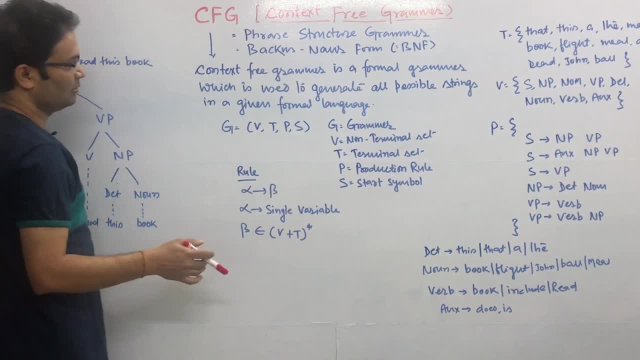 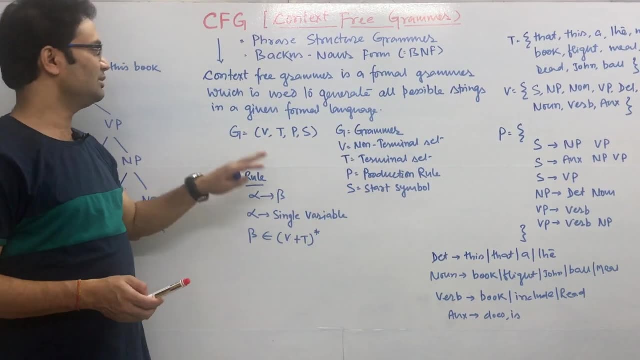 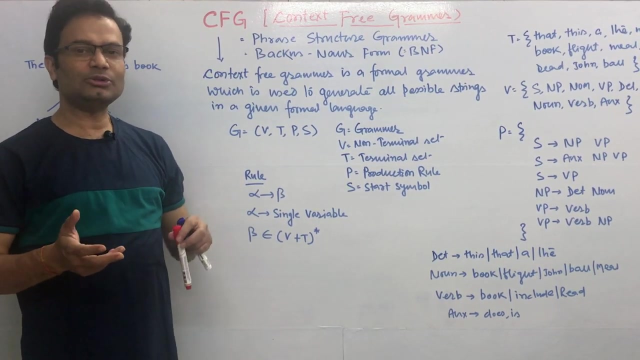 or the back-end-signal form, or most or everything are the same. So context-free grammar is the formal grammar which is used to generate all the possible strings in the given formal language. So it means that if you have any language, so your CFG should be that much of capable. 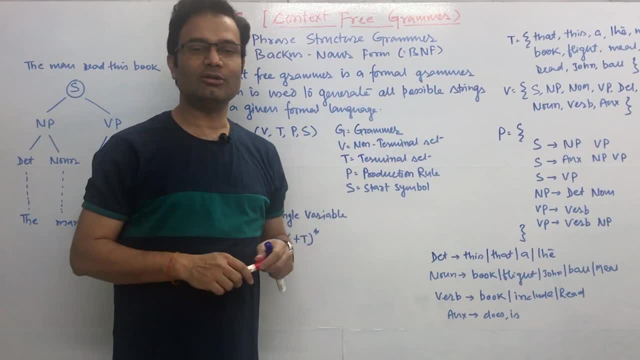 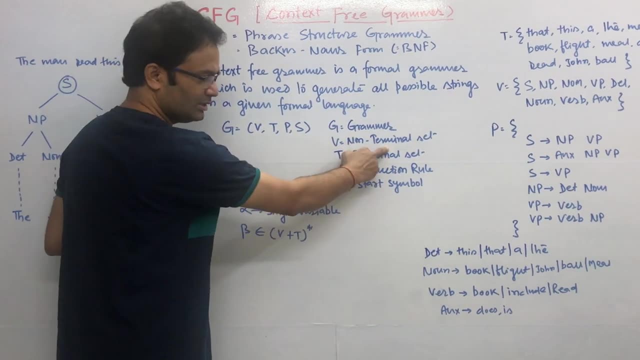 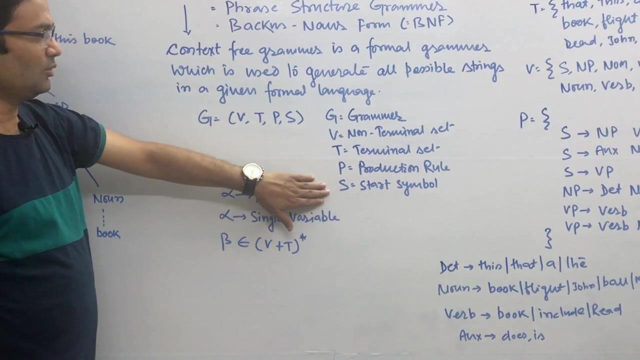 they can generate all the possible rules for the particular language right. It contains the four important part. One is the all the non-terminal set- I will explain you. and second is the all the terminal set and the production rule and the start symbol. 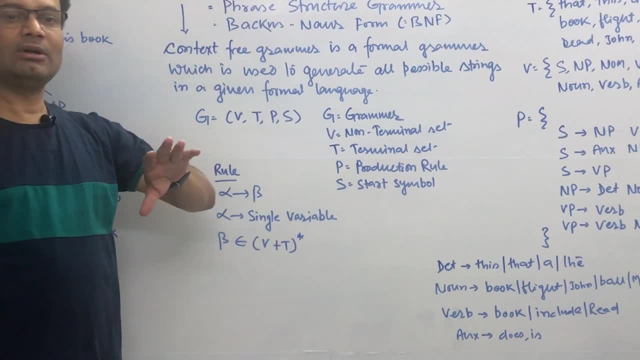 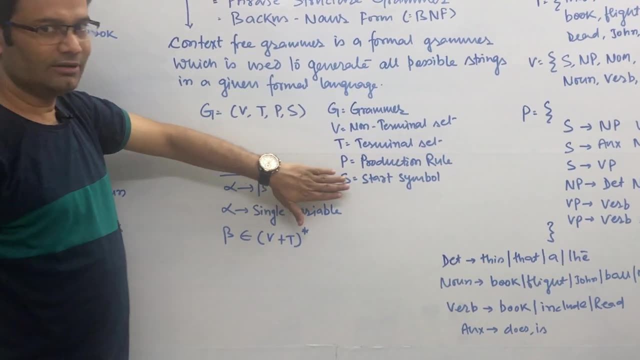 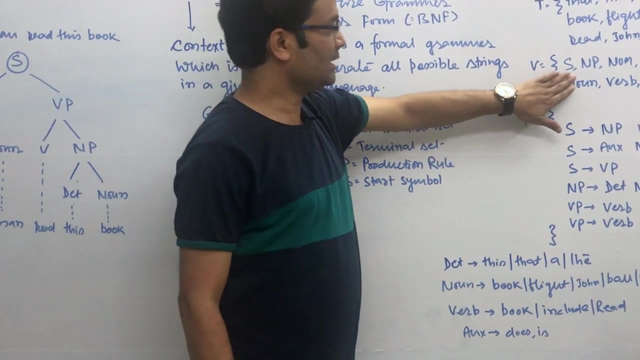 So to make one grammar applicable, or the eligible for the CFG, they should must have all the four component, right? Ok, So what is the non-terminal set? So non-terminal set could be the starting symbol, noun-phrase, noun-verb-phrase determinant. 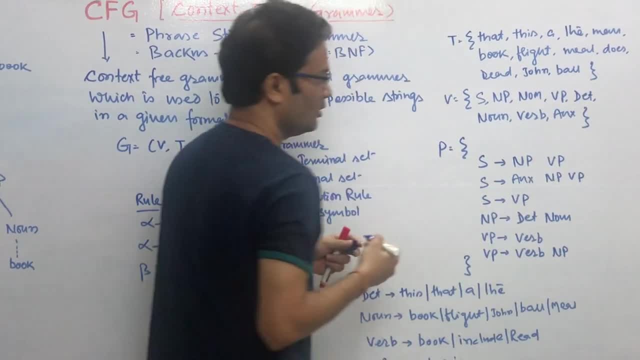 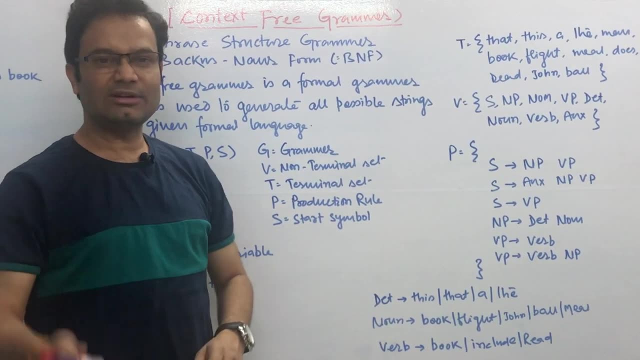 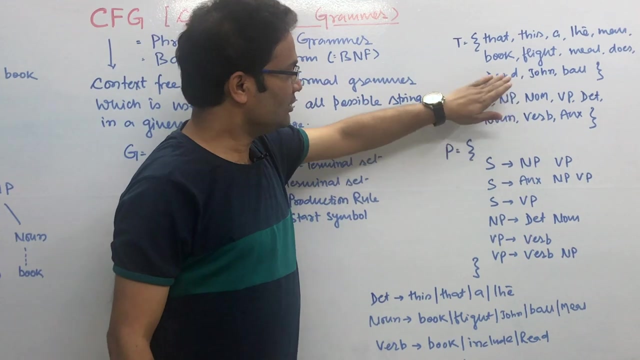 noun-verb, auxiliary-verb, and why this is called the non-terminal, when this could be further divided into the terminal. So all the phrase is the non-terminal. So when you say the noun-phrase- noun-phrase further could be divided into the non-terminal. 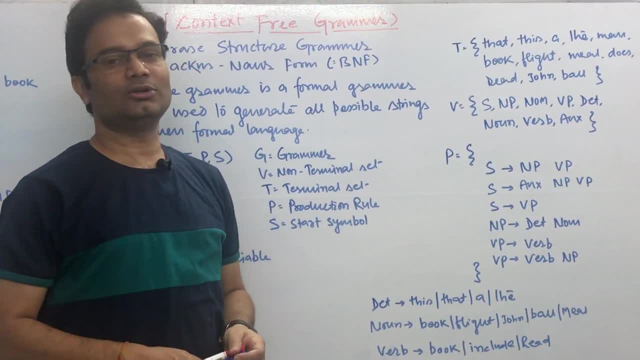 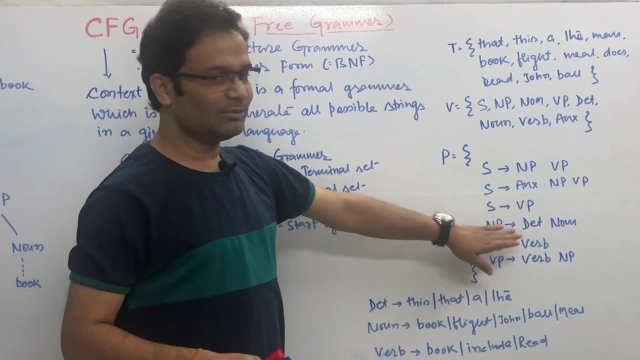 Further could be divided into the determinant and the noun. So suppose if you say the simple noun is the book, but if you say this book, so we have the determine, determinant, alt key and then the noun, So that could be further divided. 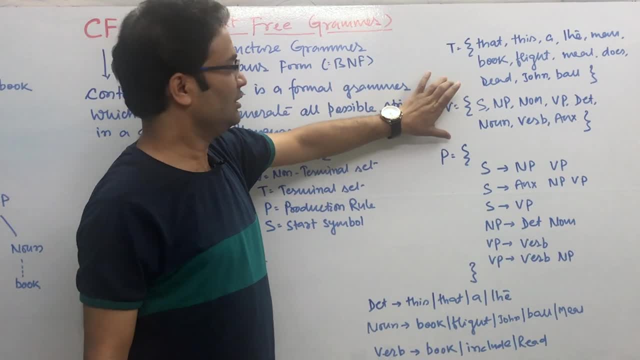 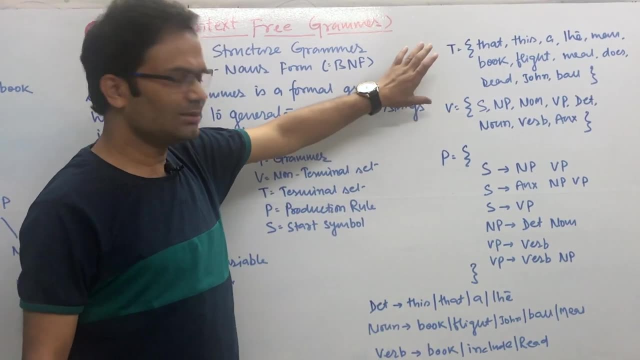 So this part could be further divided again into the terminal. So this is called the non-terminal set. We have not taken all the set, just for your explanation purpose. we have taken some subset of the set right. T is the non-terminal. sorry, T is the terminal. 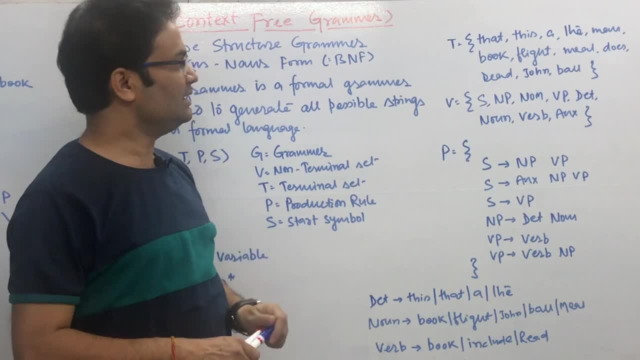 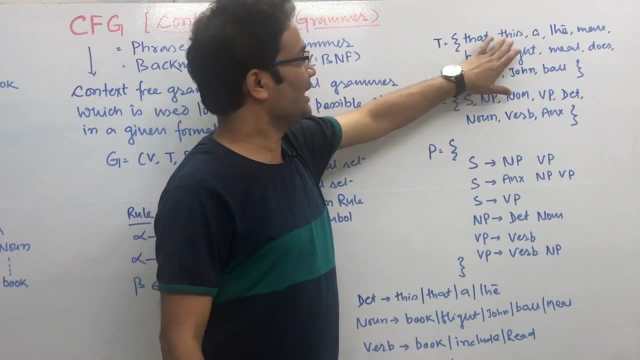 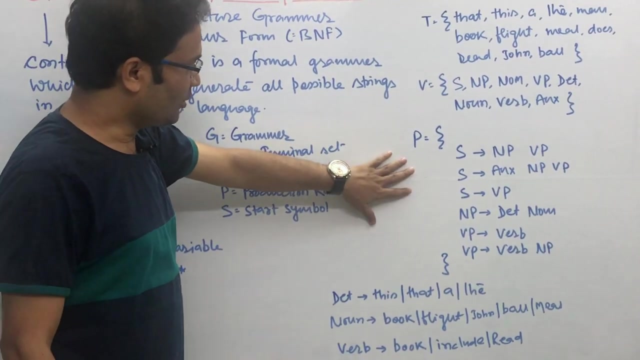 So all the word from the vocabularies is called the terminal. that cannot further divide again into the any minute parts, right. So this that a men book, right, all the English word is called the terminal part. right Now, this is important, this is called the production rule. 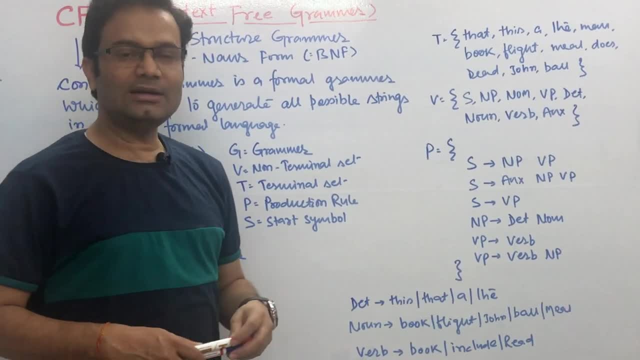 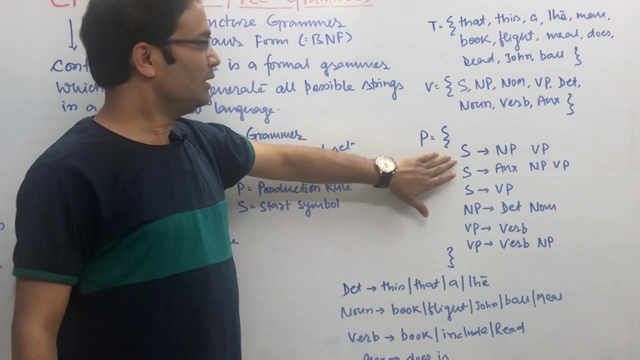 These are the rules. who can define the set of structures of the rules? So these are the rules. So these are the rules. So these are the rules for any language. So it is saying that starting symbol either could be. they contain the two part left and. 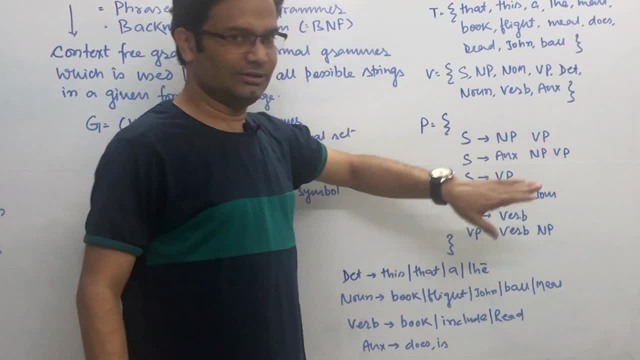 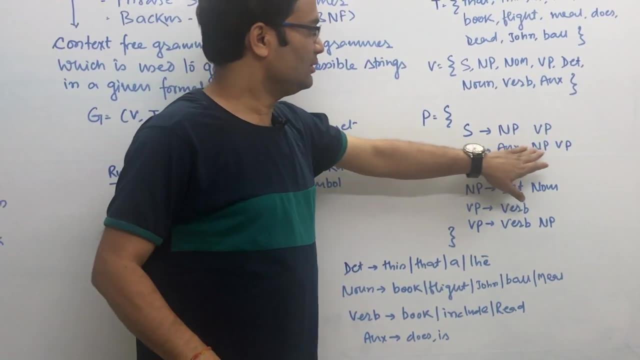 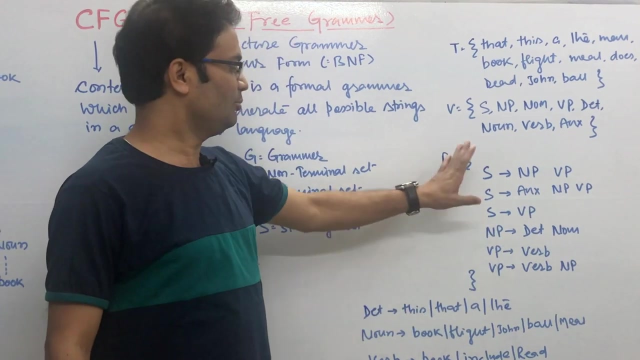 right side part: noun, verb and the verb phrase. noun phrase, verb phrase, As could be the, could have the three part auxiliary noun, verb and verb phrase. This is just a very basic example I have taken, So this kind of things could be. the production rule depend upon this, production rules we 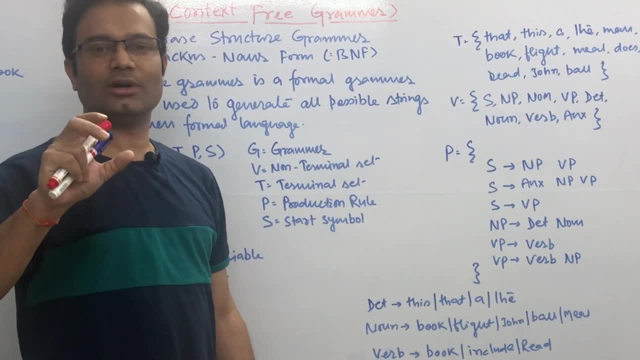 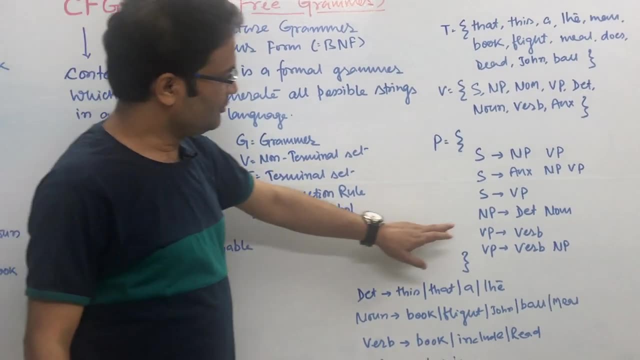 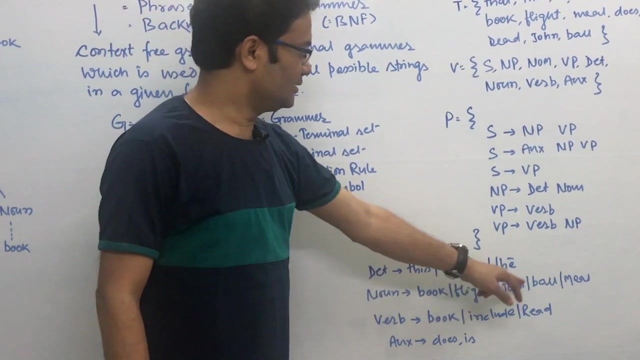 can say: So this kind of thing is correct or not according to the particular production rule of that language. right, And so I have also given that. if you say the determinant, what could be meaning of determinant? That could be this, that, a. when you say noun book flight, John, right and this. 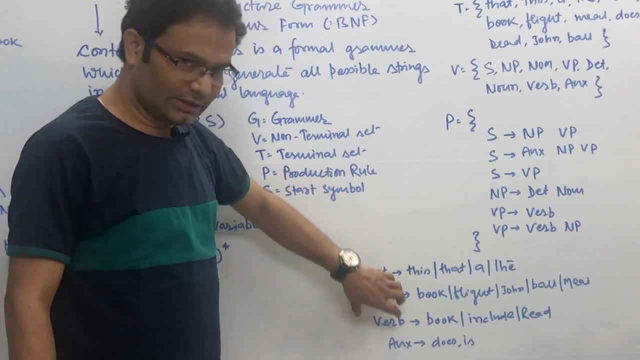 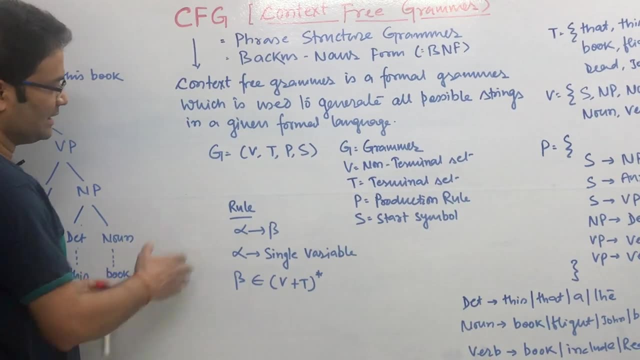 is the verb. So these are the here I have given the non-terminal and this side is called the terminal right. So, and you can also represent the CFG with this way: alpha, beta, beta, beta, beta beta. 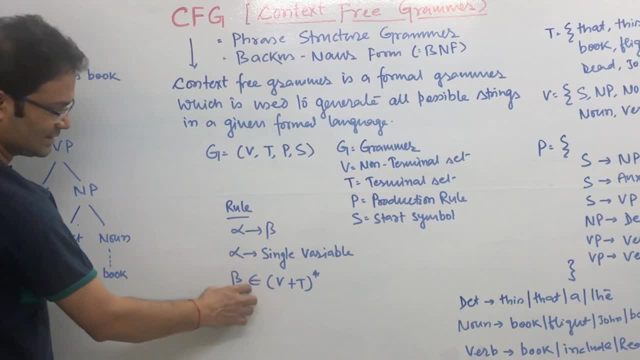 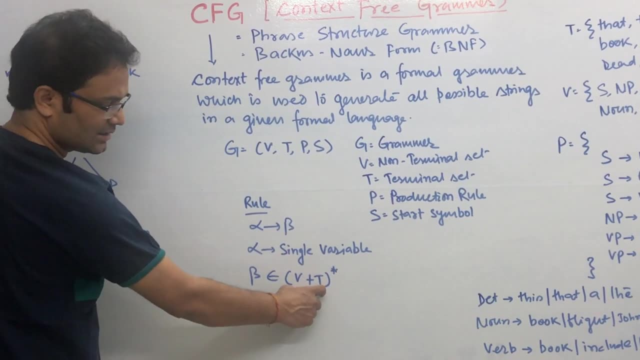 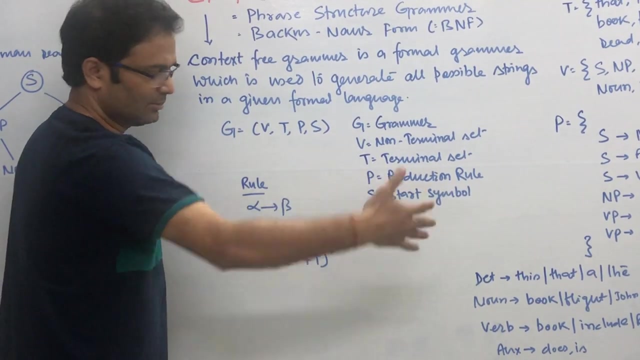 belongs to alpha, that the beta means alpha is the RSH part and beta is the RSH part. alpha will have the single variable and beta will have the combination either or non-terminal and terminal and the replicate right. it will replicate the many times. 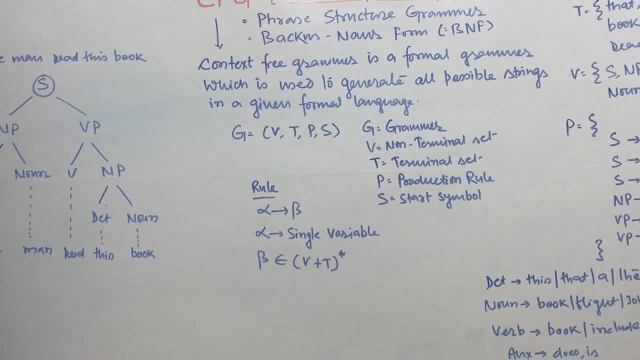 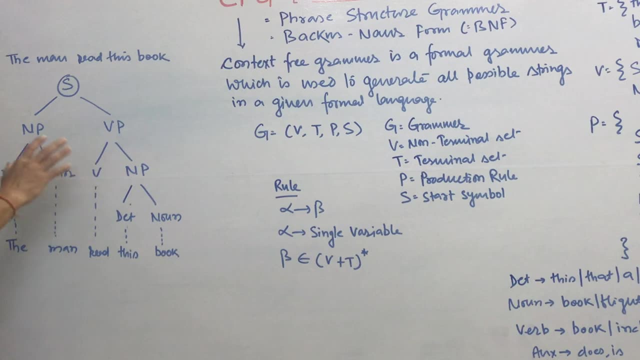 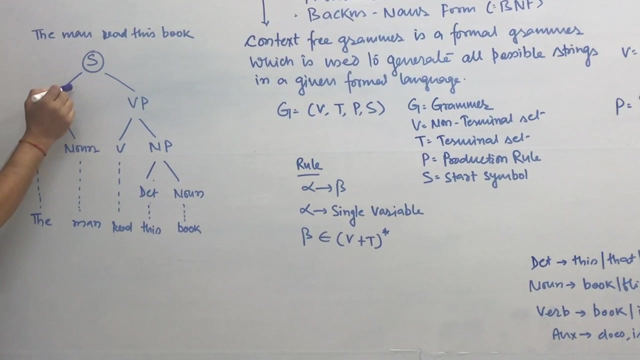 This is also one of the way to represent the context: free grammar. So suppose take one sentence- the man read this book- how to make the dish tree. So, first and foremost, This starting symbol must be there so you can start, and you can see that in this sentence. 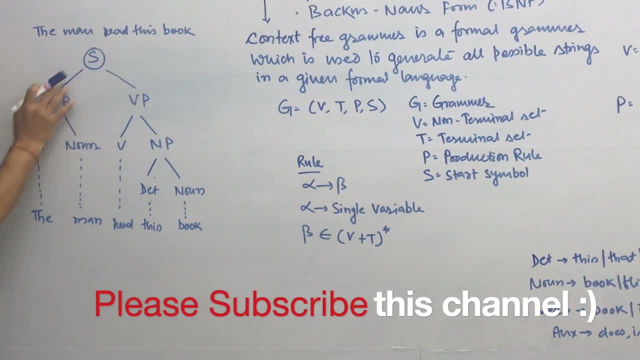 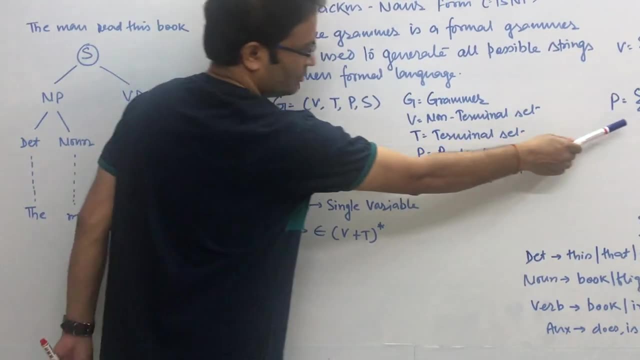 we have the noun also, we have the verb also. So take this approach, so as could the noun verb and the verb noun phase, the verb phase. So I have taken this. this rules as noun phase and the verb phase right. 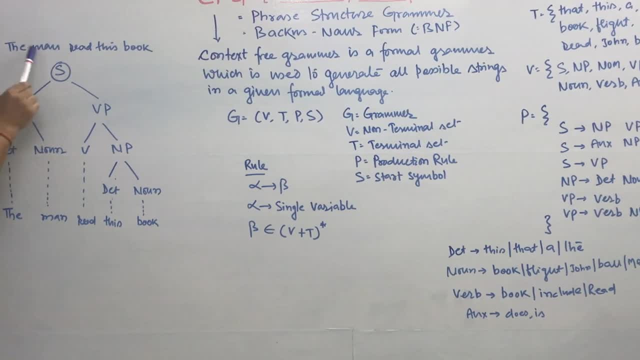 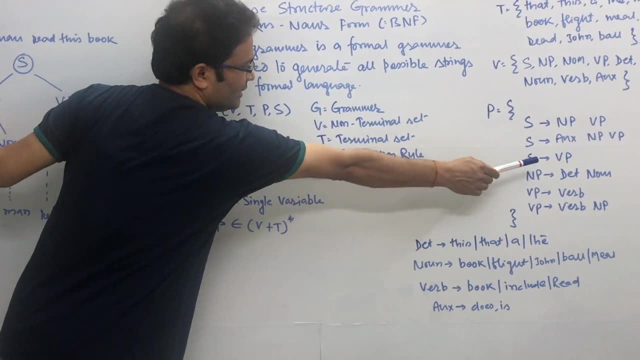 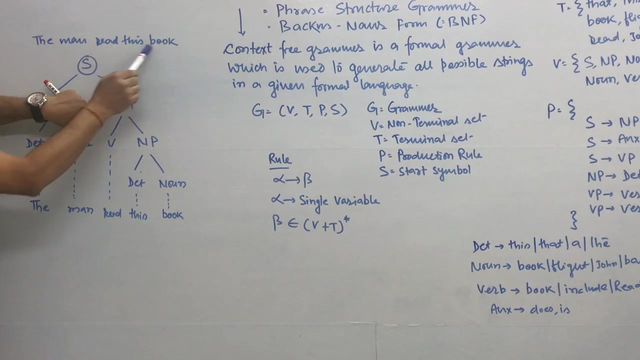 And this noun. further, we have the in the noun, we have the determinant also. so for this noun phase I have taken this rule: see determinant and the noun. so determinant and the noun And the verb, I can see that we have the one verb. one noun is also attached with this. 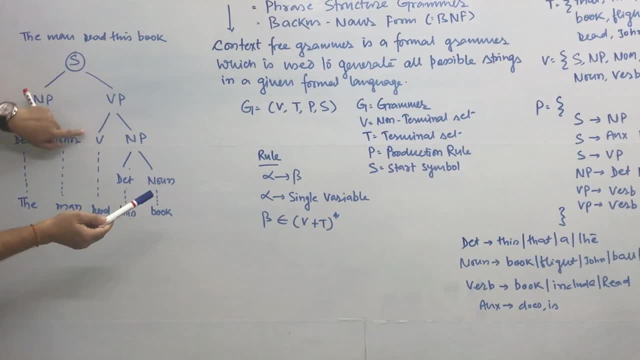 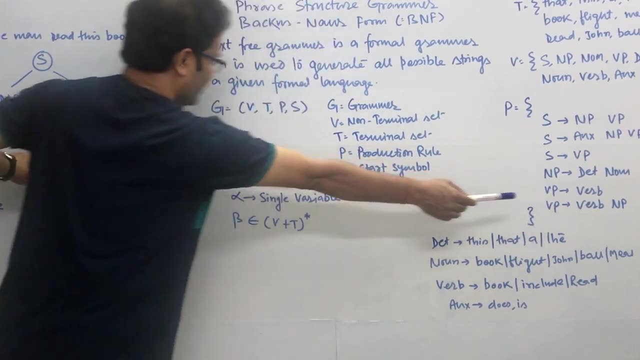 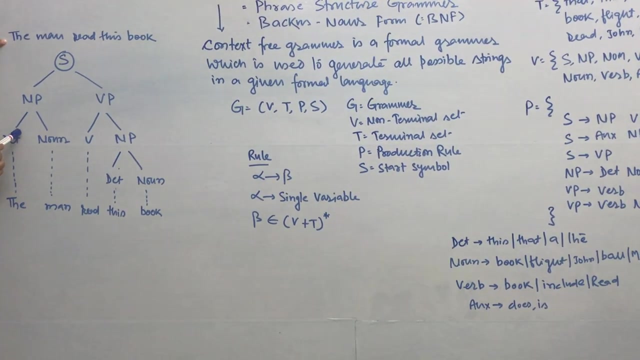 verb, right. So this verb phase further decompose into the verb and the noun. so that could we have also. So verb phase include the verb and the noun phase. we have taken this rule to divide this part. So now determinant is the, the, so here this part is the non-terminal and this is the terminal. 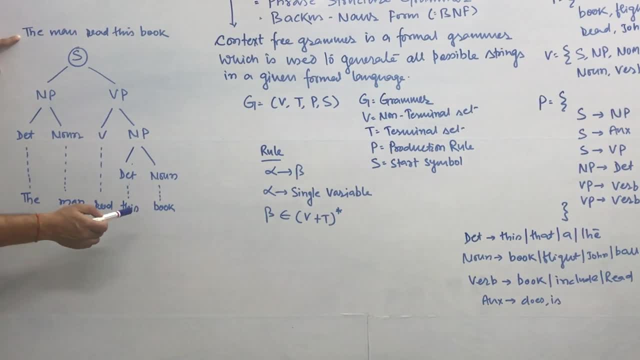 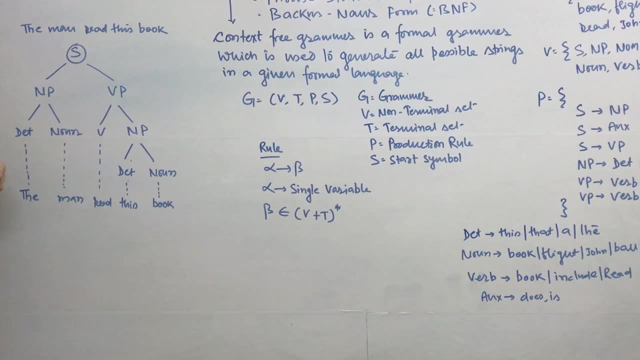 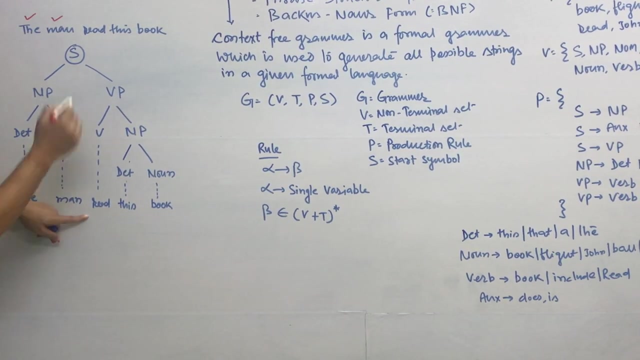 So at the end all those should be, must be terminal. we cannot left out with the non-terminal. So determinant is the noun, is the. so if you see this determinant, the complete, this noun is the main, then this verb is the read and this noun phase further divide the determinant. 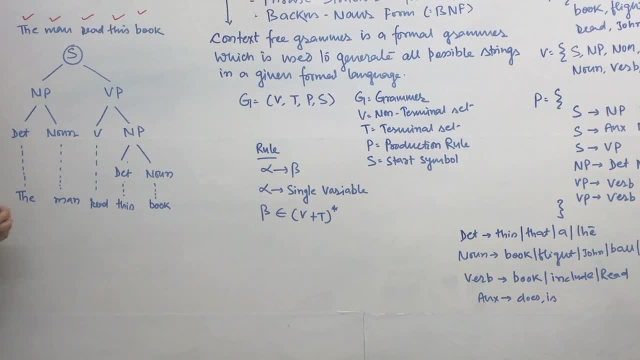 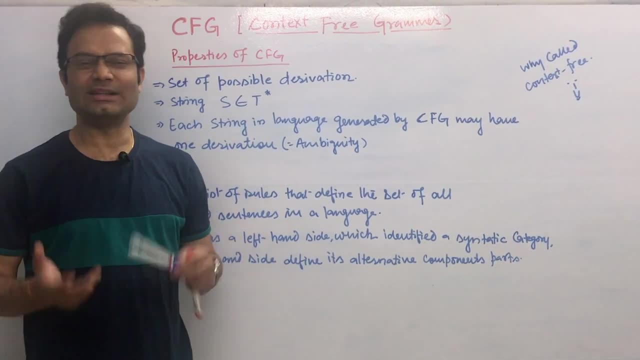 in the noun this book. So this is the way we can draw the CFG. Now discuss that context. free grammar: it does not mean that could only for the natural language processing. that could be for you any programming language also, like the C. 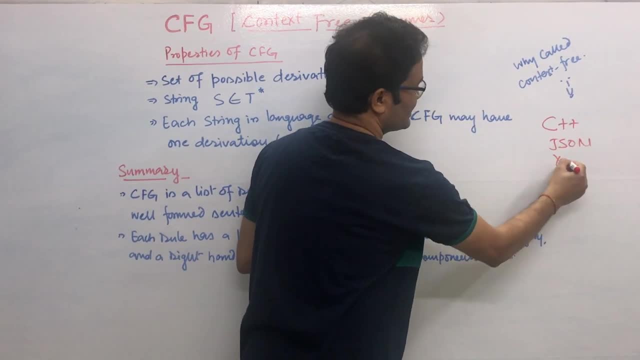 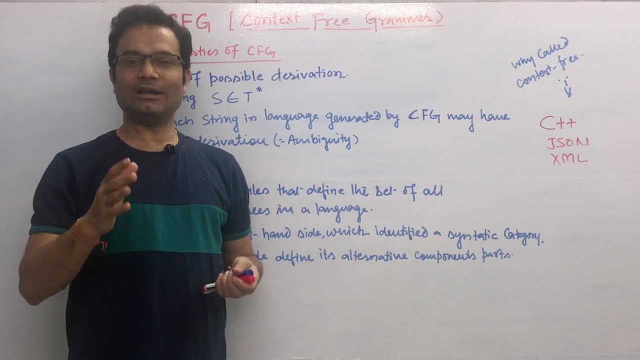 plus plus JSON file or the XML file, anything. So suppose in the C plus plus, when you write some code you must have a byte with the some set of instructions, Means when you do the programming you must have a byte with the some set of instructions. 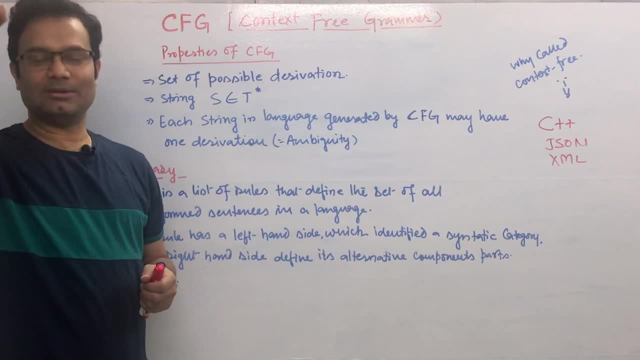 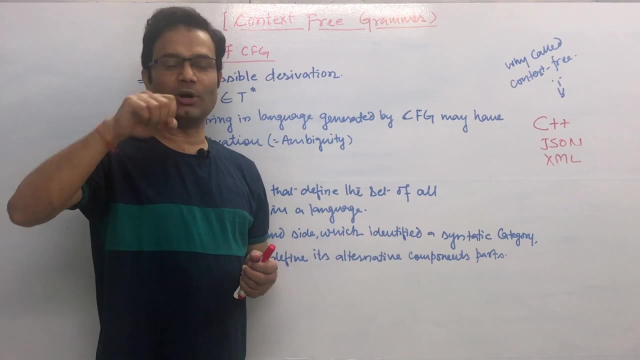 Means when you do the programming you must have a byte with the some set of instructions, So the for loop. they give some set of the mandatory and the optional thing. You cannot go beyond that right. And when you do the do while or the while loop, 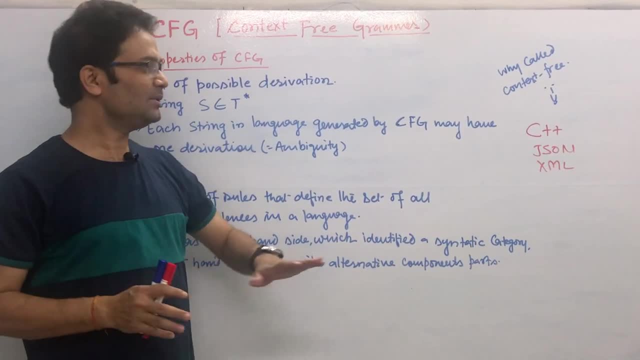 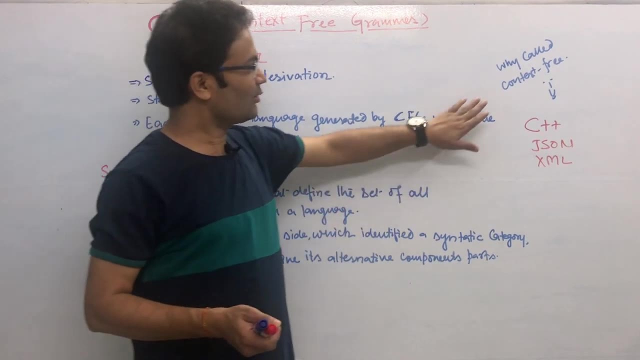 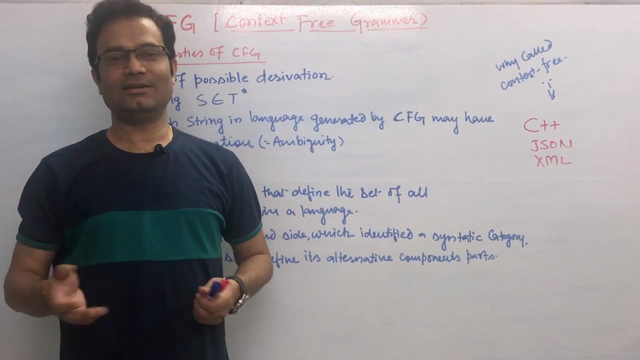 So those kind of rules has been set up in the C plus plus CFG. So accordingly we can do the R coding right And that is what is called the context free Means, suppose if you have any CFG for the C plus plus so you can write anything any. 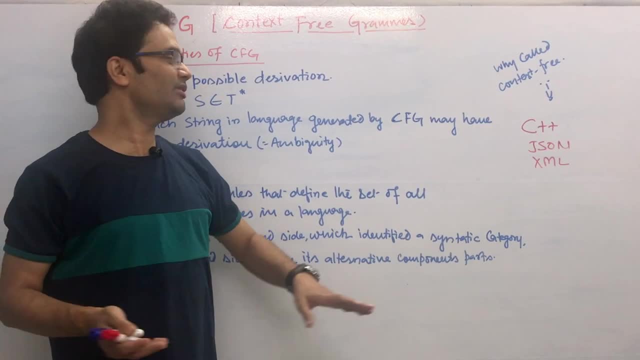 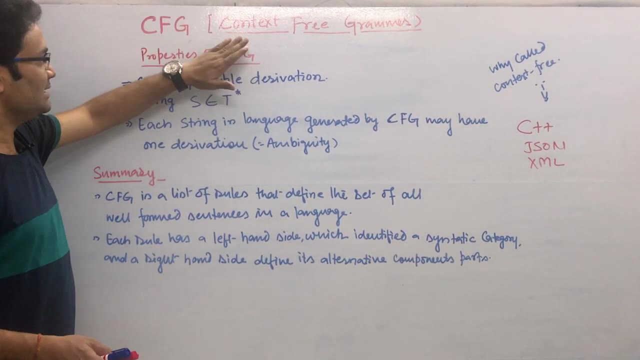 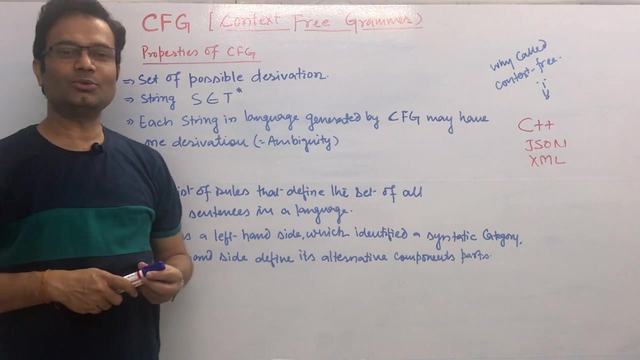 context write your code. that is the contest-free grammar. the compiler of the C++ is the contest-free. That is why here also called that the CFG. contest-free means if you take one English CFG or for any language, you are free to write any contest with the help of that CFG. that 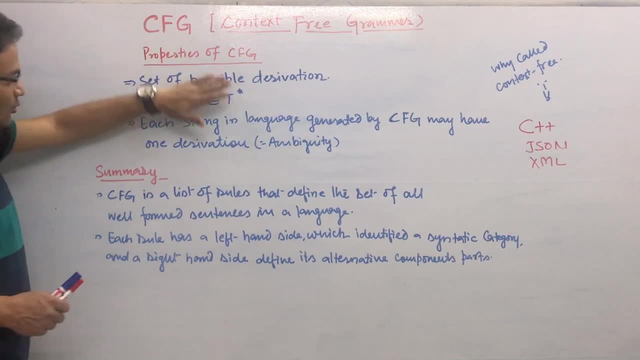 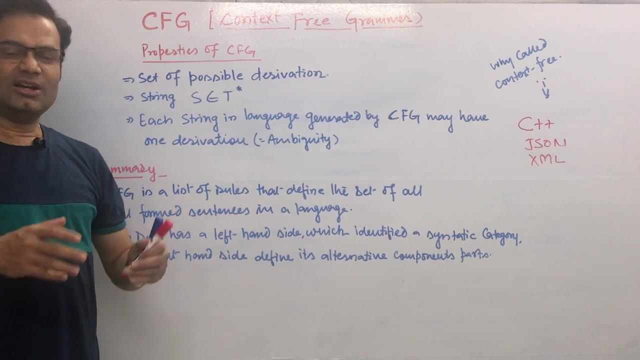 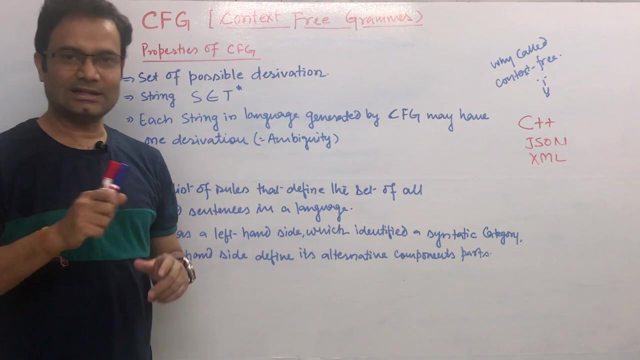 is why it is called the contest-free grammar, So we have the few properties. the same thing here means set of the possible derivations. means you can. if I set up the CFG, you can write all the possible combinations of the sentences. means all the possible derivation you can write, and string is that belongs to. 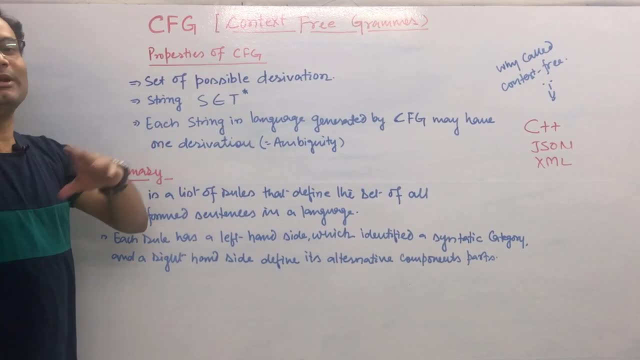 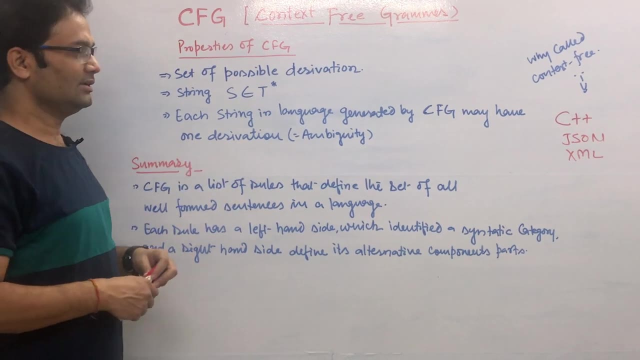 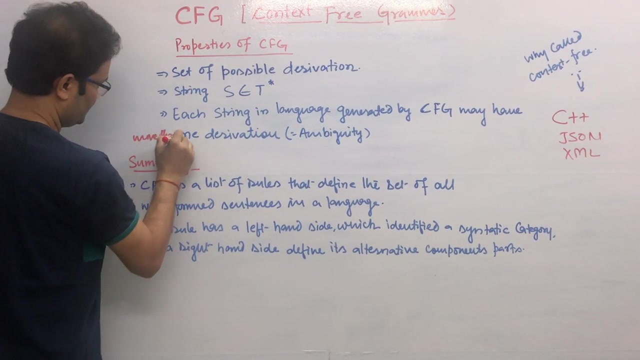 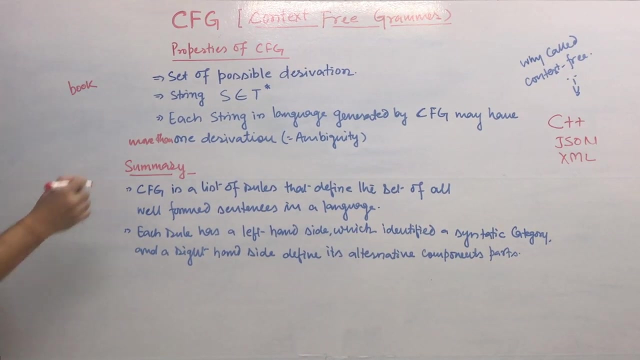 the T. So final output is the combination of the terminal things and each string in the language generated by the CFG. they have one derivation, So they may have more than one. So suppose in any sentence you have used the book. So book has the two meaning. one book is for the study purpose and another book is for 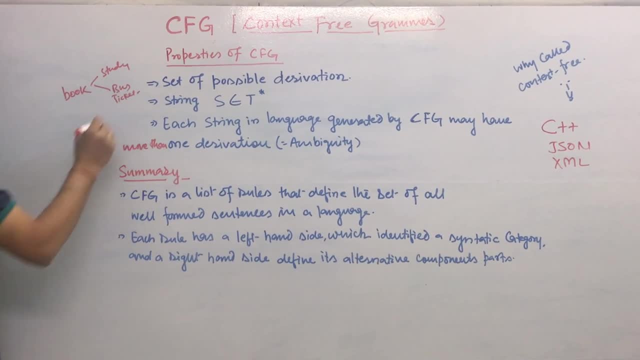 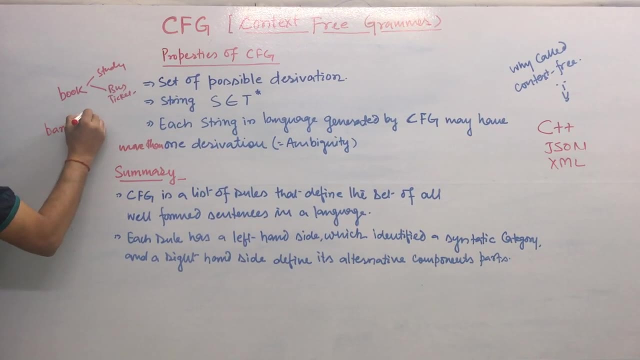 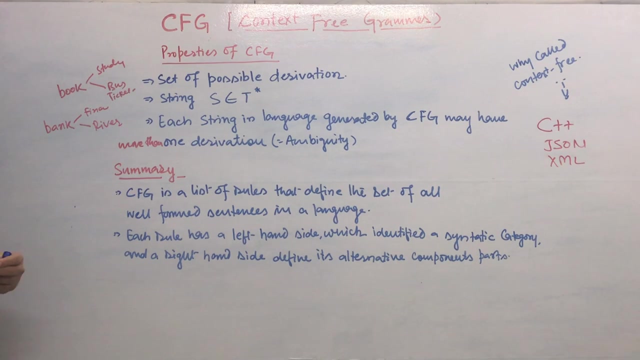 the bus or the bus ticket or the flight ticket for booking. for the both we use the book The same way. if you have the bank, bank could be the financial institutes and the river bank right. So using having this kind of the words we can generate the ambiguity in the CFG right.